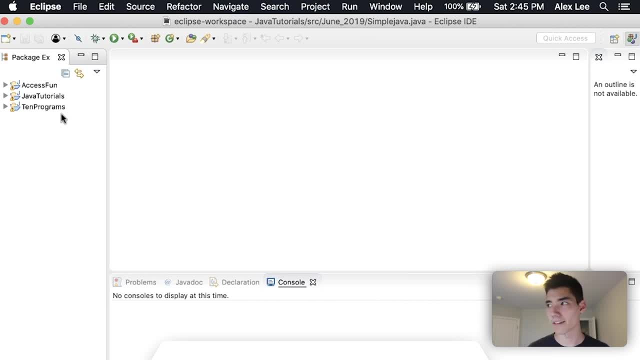 Today I'm going to show you what object-oriented programming is, And you may be in a class right now, like a Java class or doing an online course, but they may be using a bunch of fancy terms like polymorphism, inheritance and things like that, But for me, all that did was just confuse me more. 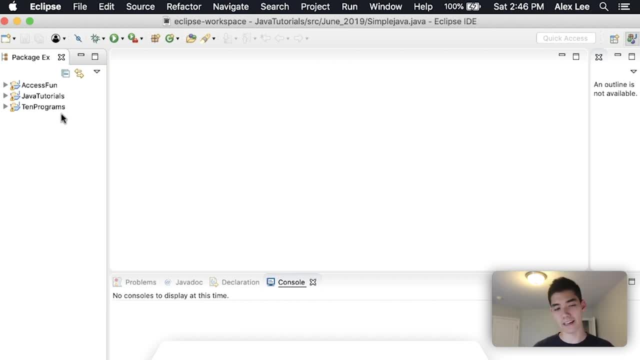 So I'm going to try to show you what object-oriented programming is in a very simple, succinct way. It's going to be my goal in this video. So, if you're new here, my name is Alex. I make Java tutorials on this channel every single week. 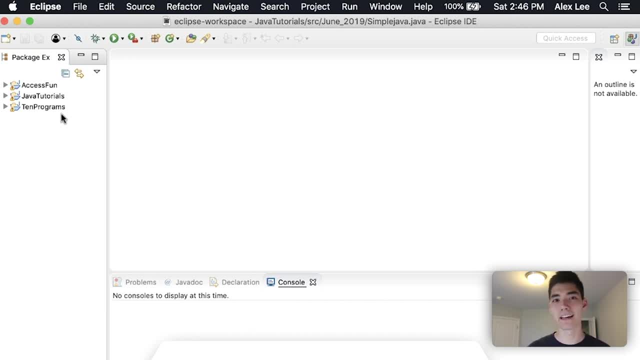 just like this one. So if you're new here and you might be interested in that, then consider subscribing. But we're in Eclipse. Let's learn some object-oriented programming while we're at it. So we're all on the same page. We'll just start a new Java. 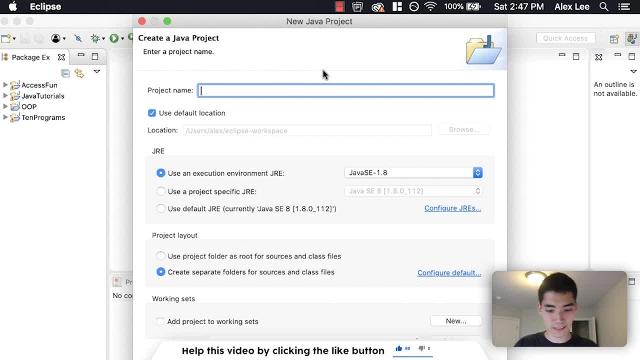 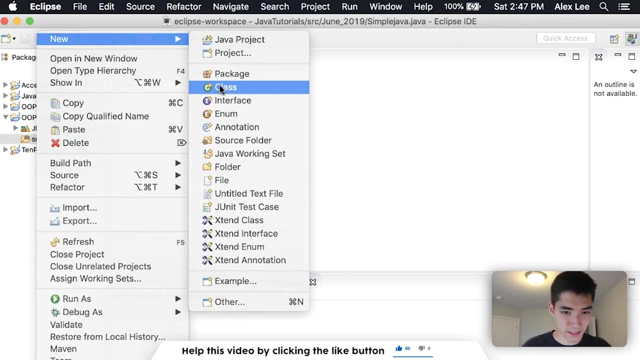 project together by going to File New Java Project. I'll just call it like something like object-oriented programming. E is fun Like that. Hit Finish And inside that Java project right-click on Source and go to New Class. This is an Eclipse-oriented program And if you're new here you might be interested in this. 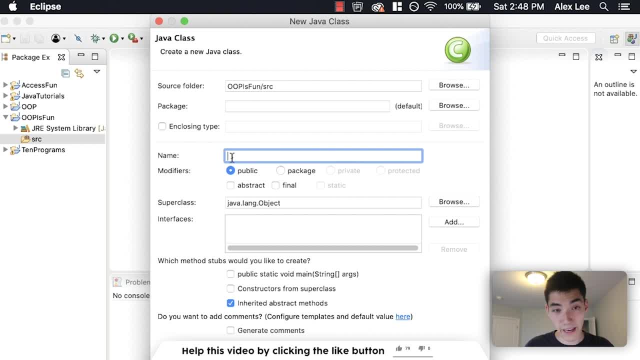 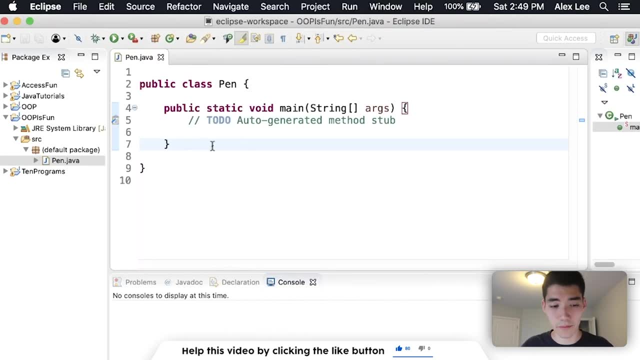 This is a Java file, So we'll just call it something like Pen. We'll call it Pen And then hit this Public Static Void Main checkbox And then hit Finish. So this generates some code for us, And we can write code inside of these curly braces, like, say, a print statement like: 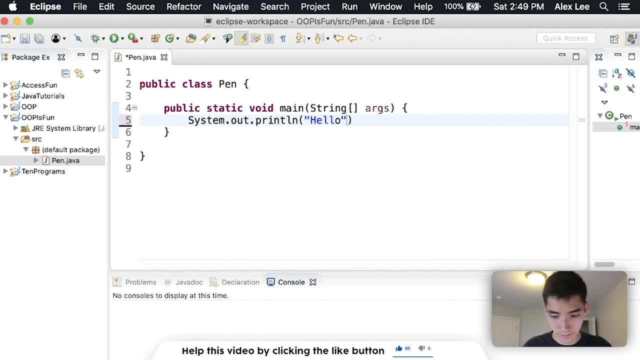 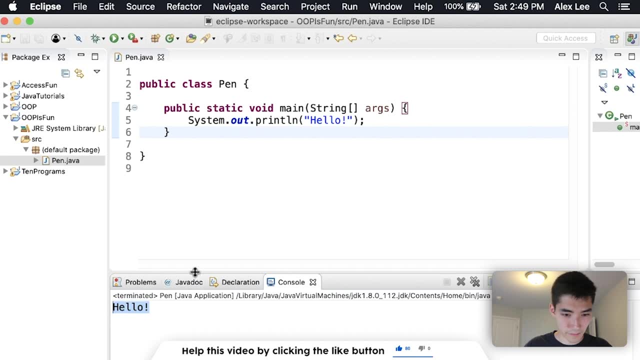 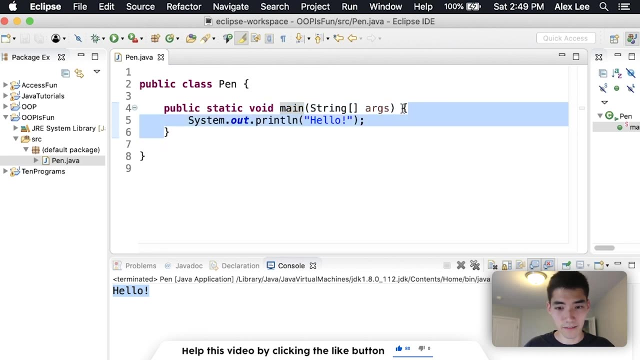 this. Let's say we'll print Hello. If we save it and run it, then in the console window down here we get Hello, Because whenever we click this green Run button that runs code inside of the main method, So anything inside of the curly braces. 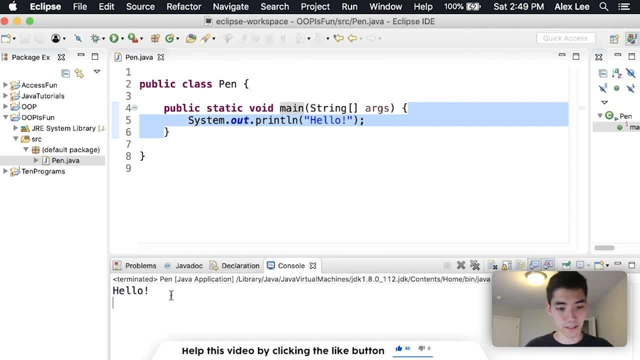 will get run when we click the green Run button And that's why it prints Hello. This print statement, for example, is just code. Any programming language has code like this. Like one line will do this, This one line will print Hello. Or we can say this one line: 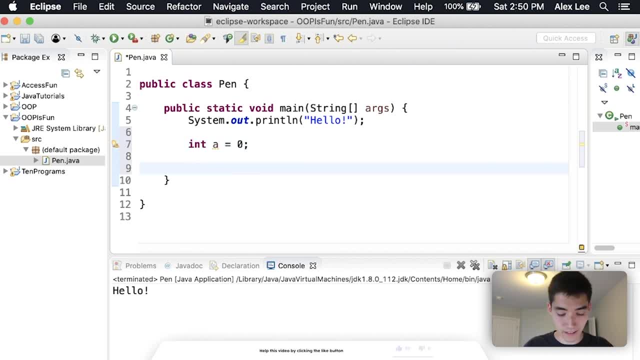 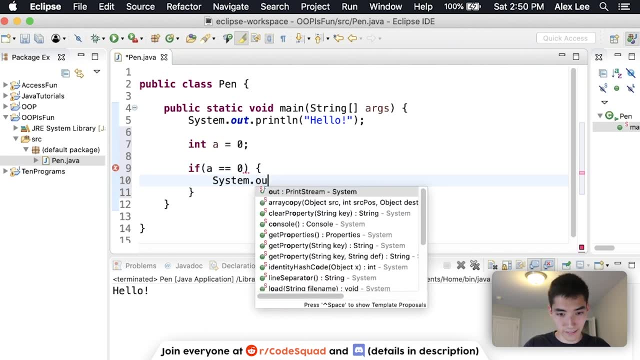 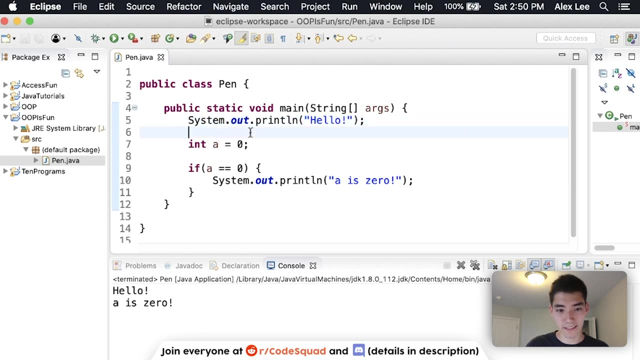 sets a variable, a equal to zero, Or even this line will say: if A is equal to zero, then it will run code inside of here. And this is all just code. It's programming, It's a line-by-line sent of instructions that 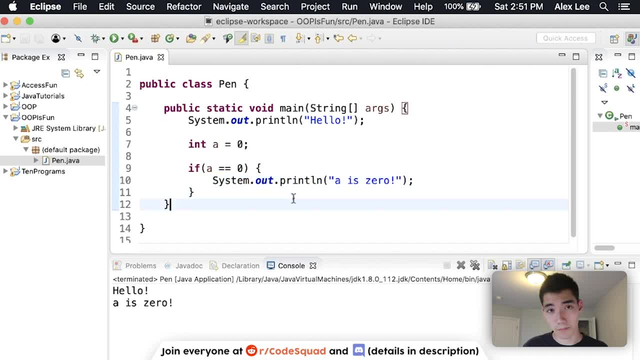 gets run, So you could do this in Python Or Java Or Kotlin or Swift or C. So we know that programming is. But what is object-oriented programming? Imagine we get rid of this main method here, So all the programming inside has got. 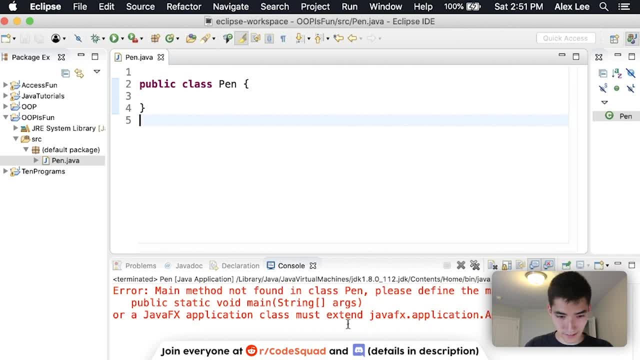 gone and we tried to run this. we get red text. it says error: main method not found in class pen. whenever we click the green run button, anything inside of the main method gets run. and since there's no main method, nothing runs and we get an error. so right now i want you to forget everything. 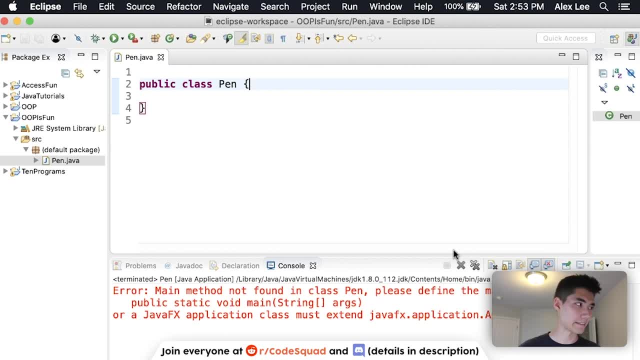 you know about a main method or programming. don't try to memorize any of what i'm going to say, just kind of follow along on your phone or on your computer. i've got a pen here. it's a blue, blue pen, um, it's pilot g2 and it's 10, 10 point. i think that's 0.1 millimeters. 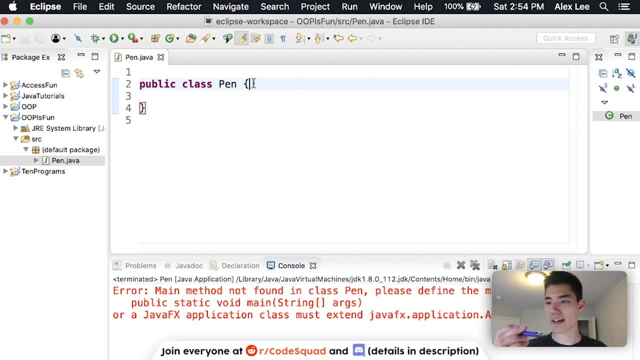 it can click and it's a gel pen. i think it would be pretty cool if we could turn this real life object that is blue, that clicks, that i can physically write with what, if we could represent this inside of a computer. i think that would be a pretty cool thing to do. so i'm just 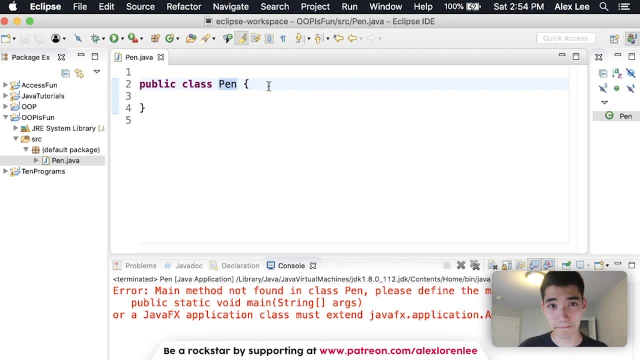 gonna show you how we would do that. we already named it pen and we'll just start describing it like. what is it? well, it's a pen. it's a gel pen. so we can say: like type is gel. like that we can say: the color: the color is blue, blue it's. 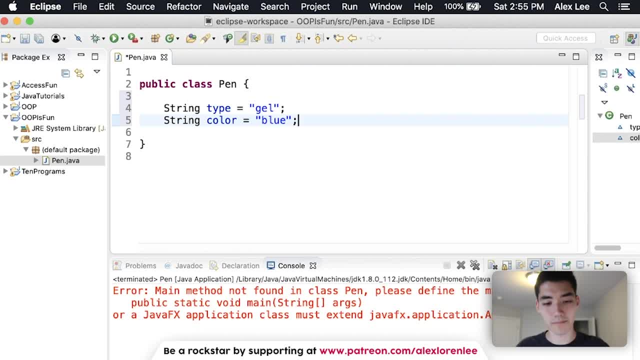 a, it's a 10, that's the point of the font. so we can say: points is 10 and that's it. just a few things to describe the pen. it's a gel pen, it's blue and it has 10 point. well, now we've sort of described this pen inside the computer, this real 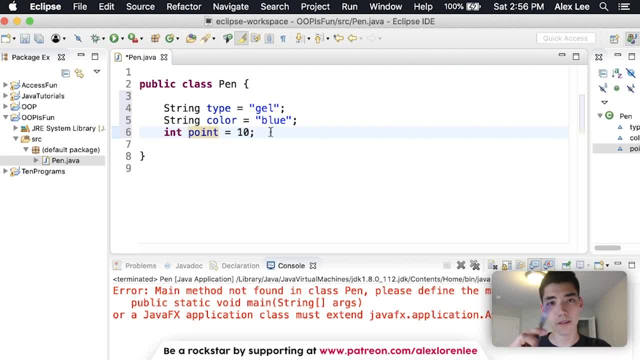 physical pen inside the computer. let's think about some actions we can do with this pen. well, it looks like we can. we can click it, um we can, um we can, and take it apart, like we can untwist it and maybe replace the ink tube inside of it. 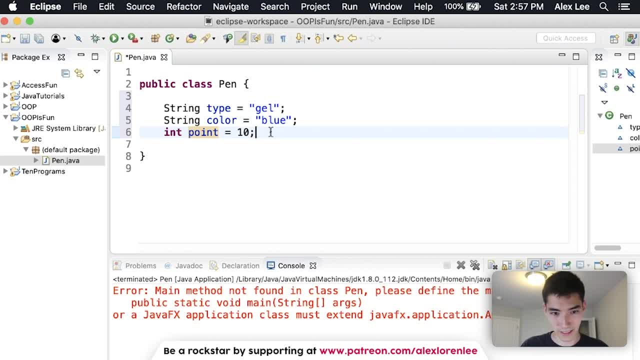 So let's try to describe those three actions in here. Well, we can write a method for each of these. So one thing we can do is just write some keywords for starting off a method. We can say click, so we can click the pen. 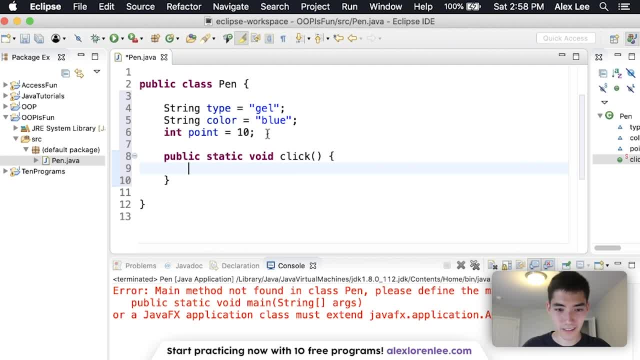 and maybe create some Boolean variable to say if it's clicked or not up here, So we can say clicked equals false, but when we click it we'll set clicked equal to true. Add the keyword static up here. We can unclick the pen. say unclick. 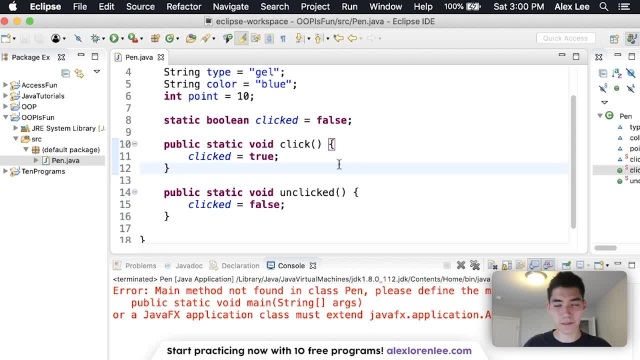 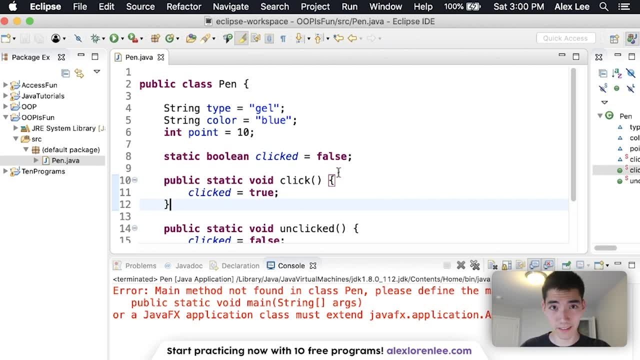 and then set clicked back to false and that'll be fine for now. So we've created our physical blue 10-point font clickable pen inside of Java. Now we can actually use the pen we've created. So to do that, we'll just make a new class. 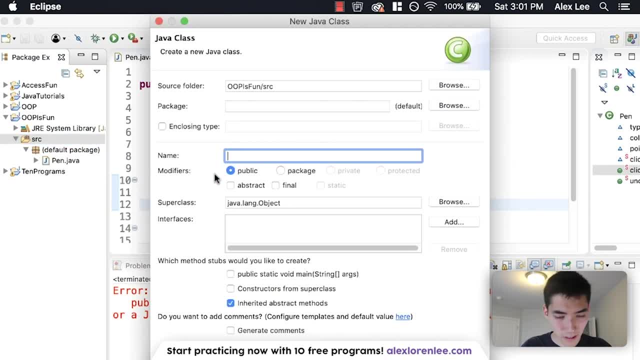 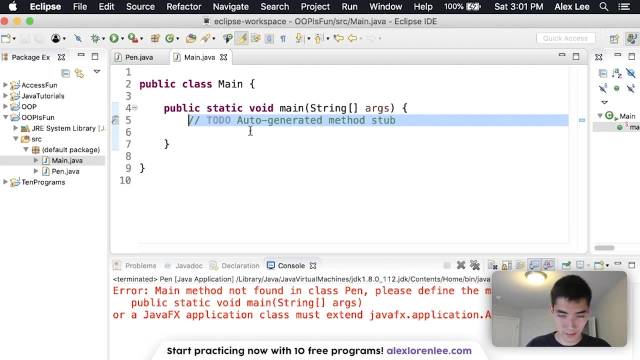 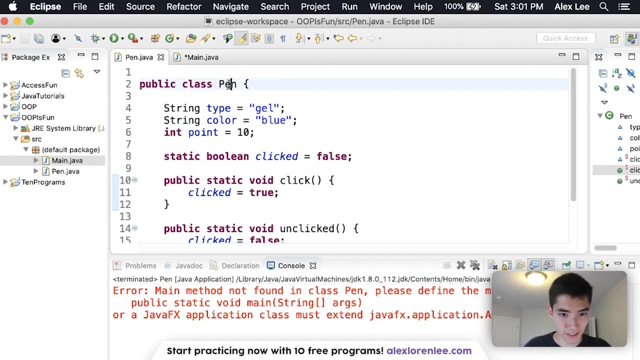 on the source folder. So go to file new class and we'll call this like main, like our main method class where we call our pen code. So to use the pen from the computer we just type pen, which is the name of our class, right here. 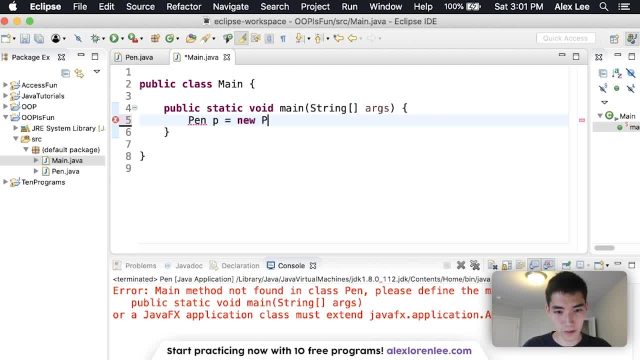 So we do pen. we'll name it like: p equals new pen. Since this is in the same folder as pen, we don't have to import it. If it was outside the folder, we'd have to hover over it and click an import. 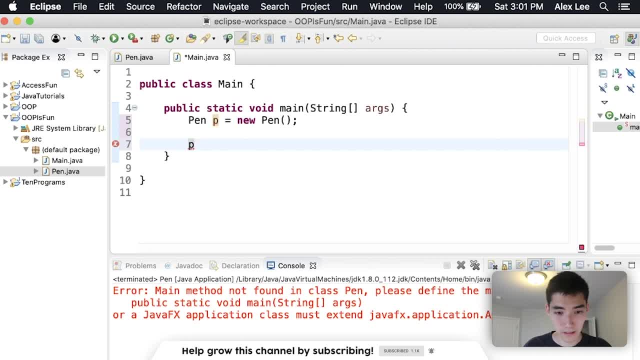 to make it work. Now, when we type p and then put a dot, the dot brings up everything that this pen can do, So it actually shows us that we have a color, a point and a type for it that describe the pen. 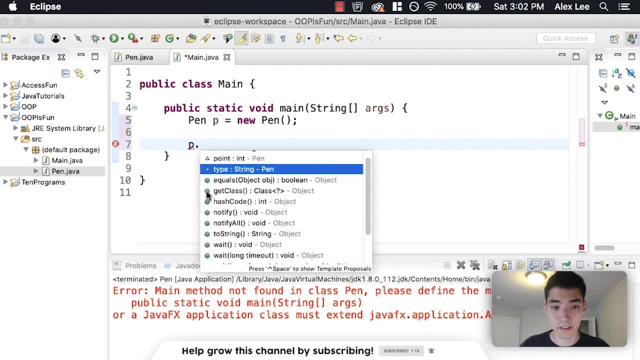 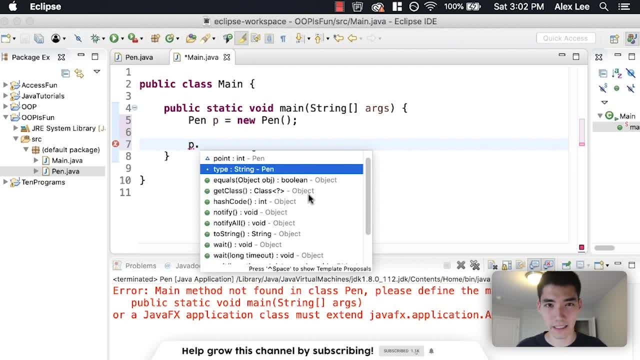 Equals, get class and hash code. These are all built in, so any class that you make will have these default methods. But if we scroll down a little bit we can see click and unclicked. Actually, that should be unclick, not unclicked. 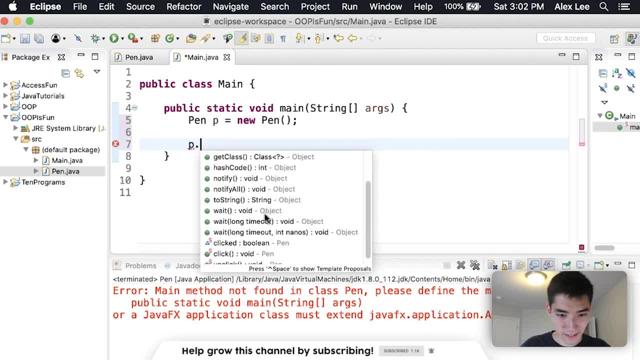 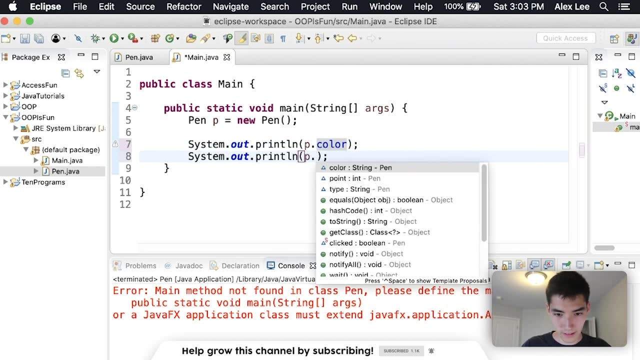 Just like that. So when we do p dot again we can see click and unclick, So we can just print out some of the attributes. So say we'll print out the color. Put that in a print statement, The color say we'll print. 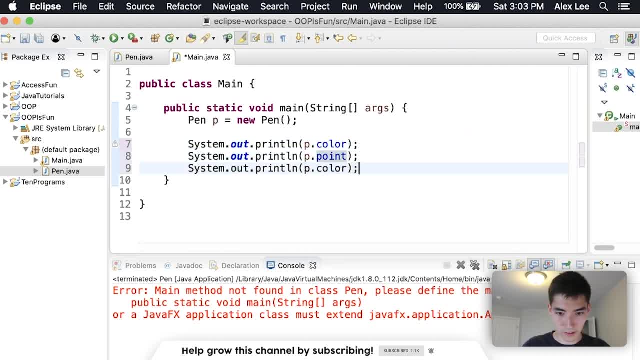 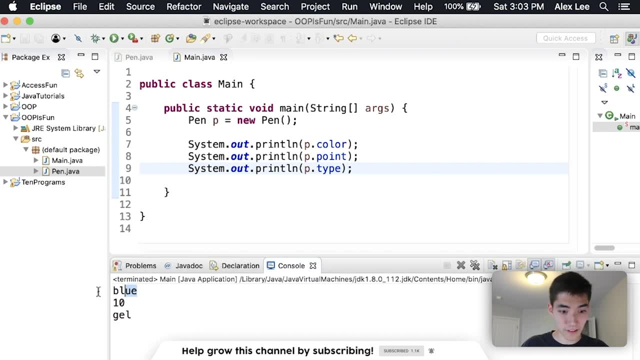 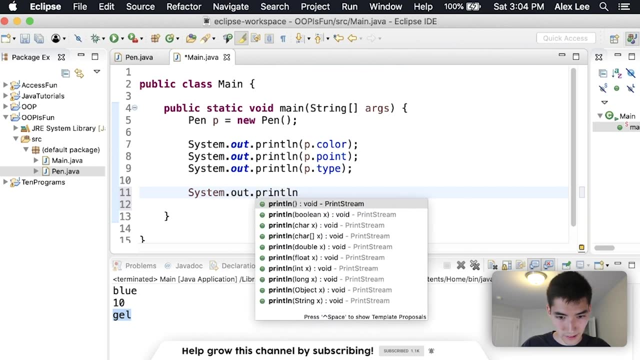 Let's print the point and also the type. So these are our three attributes of the pen. Now let's see whether the pen is clicked or not. Let's print out p dot clicked. This is the variable. Let's see if clicked is true or false. 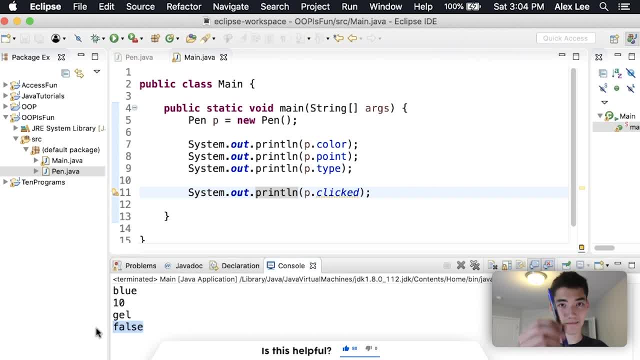 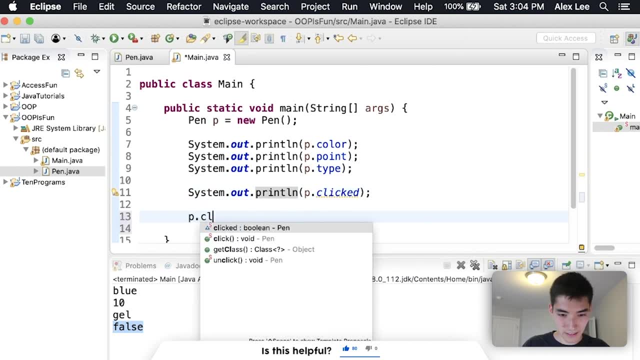 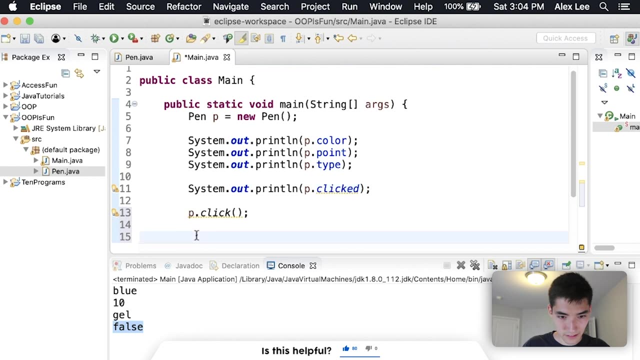 We'll run it and since it's just how it was, it's not clicked, so clicked is false. But if we run p dot click to click our virtual pen and then we print out clicked again, then we'll see that it's now true, since we clicked it. 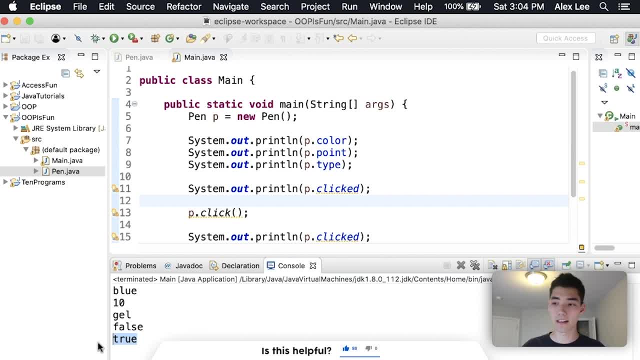 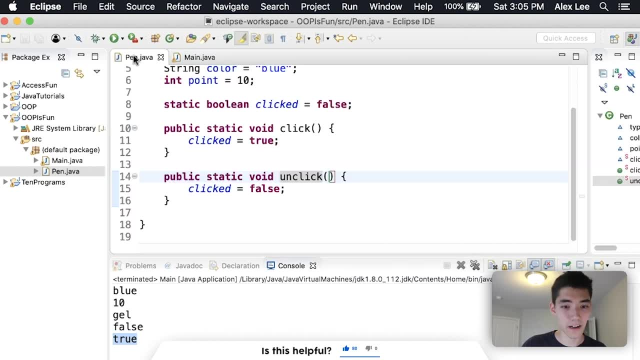 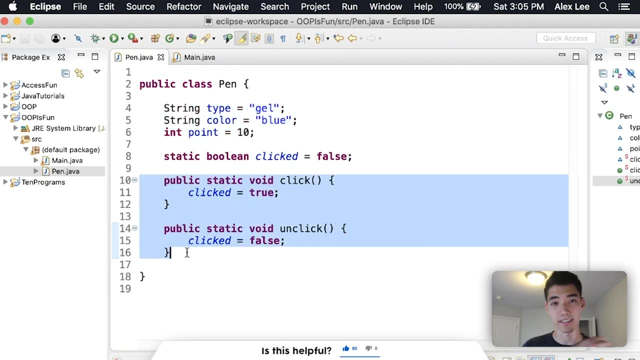 It's clicked. All object-oriented programming is is taking real physical objects or making up objects that will help you and putting them into the computer. just like this. An object has attributes and actions. It's a gel pen that's blue and .10 font. 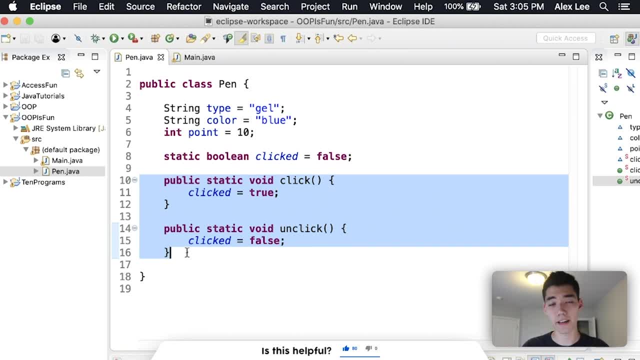 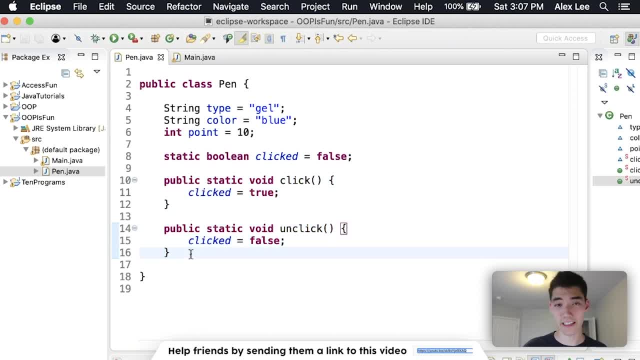 you want for your specific purpose. you can create as many objects as you want, and you can even say that objects are related to each other, so you don't have to reuse code. so say, I have this pen class, but I have three different pens here. all of them are pens, all of them well, these two can be clicked, click. 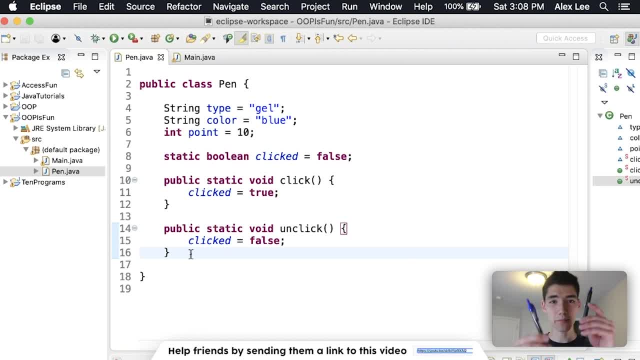 click, but this one you have to twist, so you can modify objects based on how specific you want. or you can make like a generic pen, say like it's got ink in it and it can be opened, and then you can create different pen objects that inherit or take attributes and method from the generic one and then specify it. 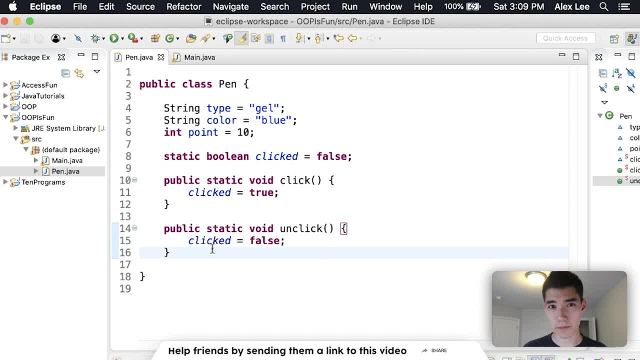 further. there are lots of different terms with object-oriented programming, but I want you to get the base, because it's really gonna help you a lot in the future if you know the very core of it. like me, I didn't understand the core of it at all, so I was trying to memorize all these different terms that I didn't. 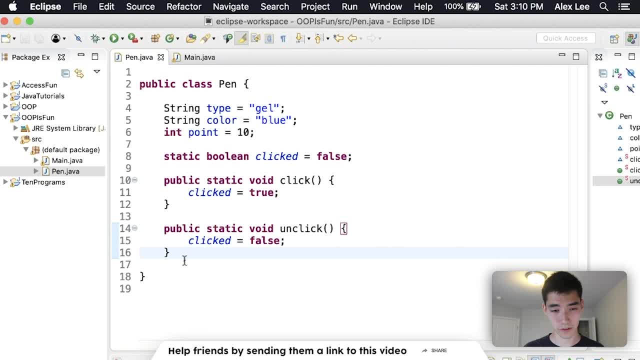 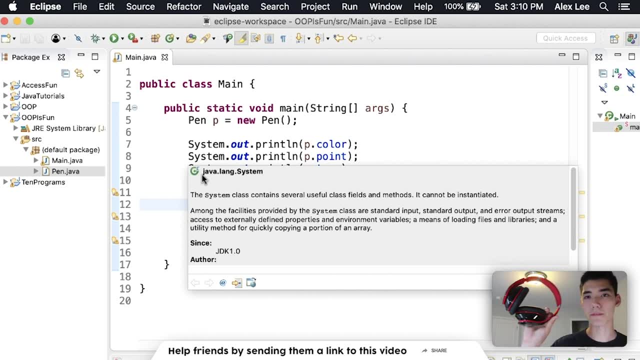 know how they related and I couldn't keep up with all these different terms. so let's do one more example. let's say I have a pair of headphones right here, a pair of headphones. they are over-ear headphones, they're Bluetooth and they're red and black. we're gonna do. 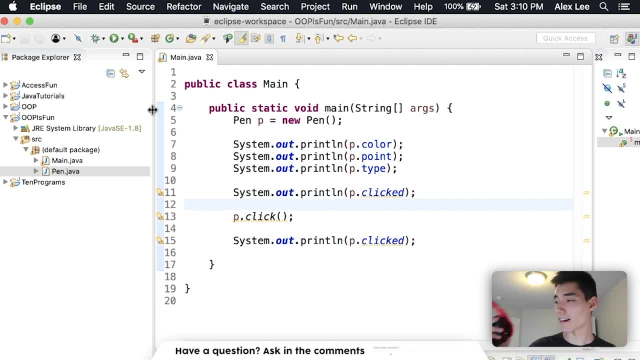 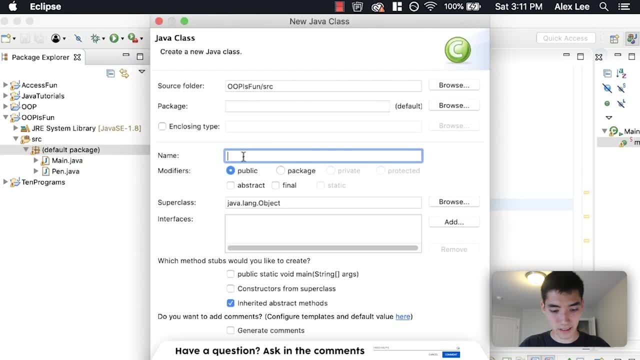 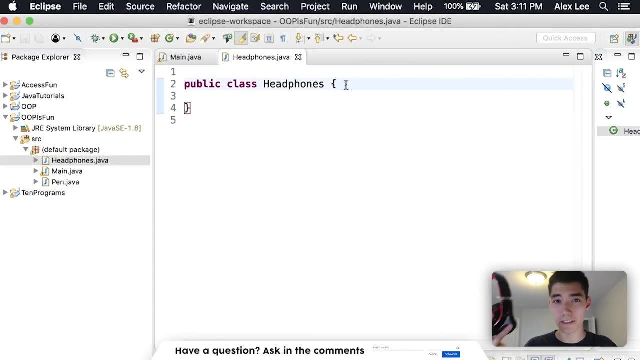 just what we did before. but we're gonna turn this physical pair of headphones into an object in Java, so we'll go to a new class, call it headphones, and hit finish. and the reason we want to turn this physical object into code in our computer is so that we can know. 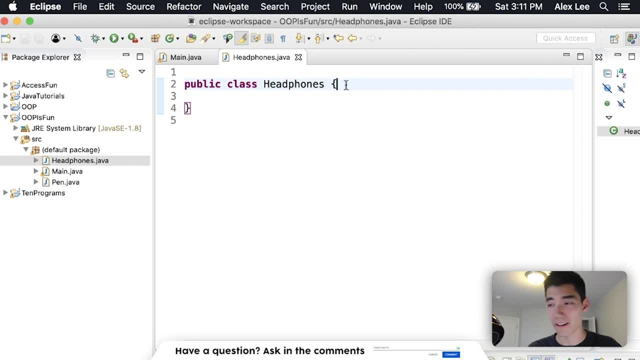 information about how these work and what they are, without having to physically be here and like. look at it. like on Amazon, there's a bunch of information you can know about this. if you're looking to buy something, there's a bunch of buttons here if you're going to buy something you might want to know. 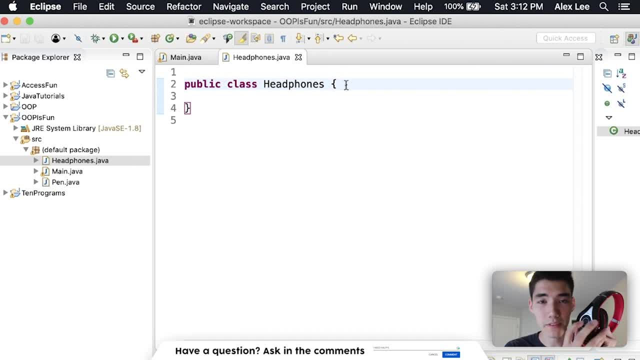 what functionality this has on the headphones. it's got volume upside skip buttons. you can take calls with it. it's bluetooth, it's micro-usb. If you didn't know any of that, then you might not know if this is the right fit for you. 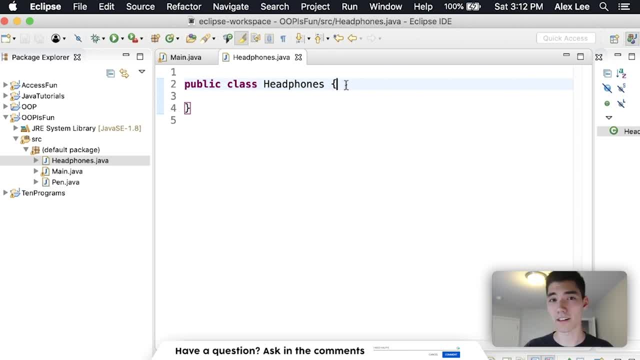 So we represent this as an object in the computer so that we can understand what it is without physically having it. I hope I explained that well, If I didn't, please leave a comment and maybe we can all come to a conclusion. So we'll give this a few attributes here. 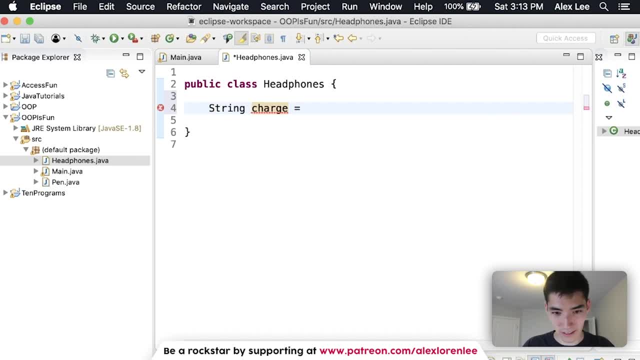 Like say the charge is a micro USB. Micro USB maybe it has an array of controls on the side- And say we can do power it's got volume, skip it's got play pause. And last we can say color is red, black. 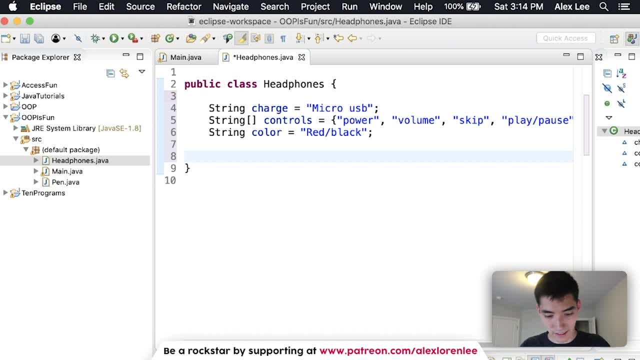 Now, what actions can we perform on this? Well, we can like turn it on, Power on, And to keep track of whether it's on or off again, we can just do what we did last time: keep a boolean variable. We'll set it to off and call it power. 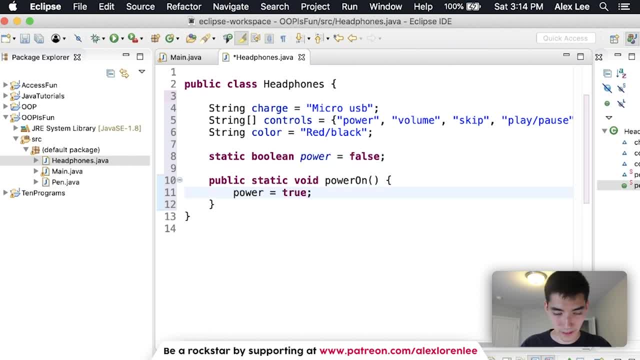 If we power it on, then power will be true. We can power it off- Power equals false- And say maybe we can volume up, volume down. We'll set the start volume to say zero And we'll do volume up Each time the volume up button is pressed. 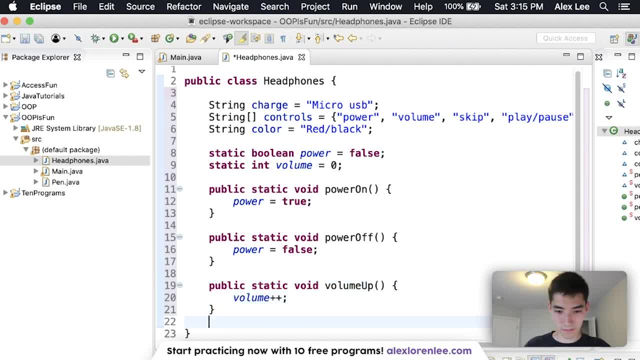 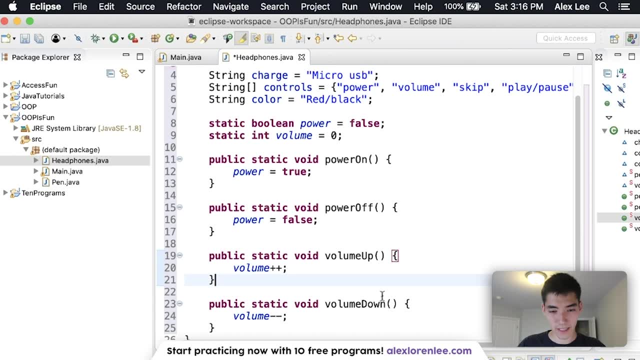 then we'll take the volume and increment it by one And the same for volume down, except each time we hit the down button we'll take it down one And we get set like max volume, min volume, things like that. But for simplicity's sake, this is what we'll have. 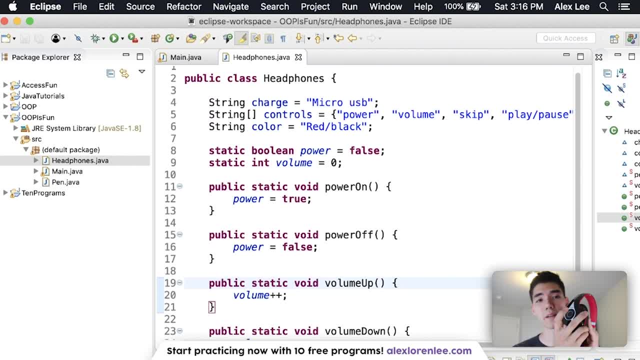 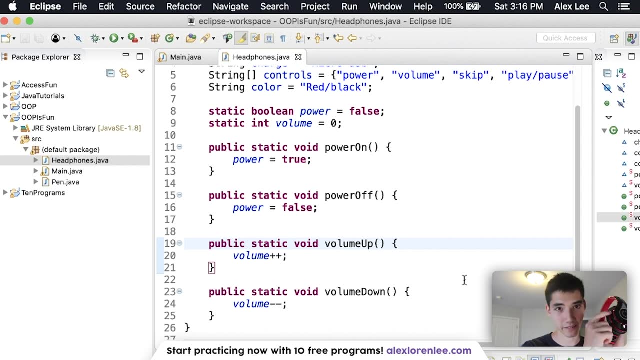 And this is how these headphones are actually programmed. Each time a button is pushed, the microchip inside of it gets the signal from one button push and then calls the volume up method or whatever turns the volume up inside of. here. It keeps track of these different states. 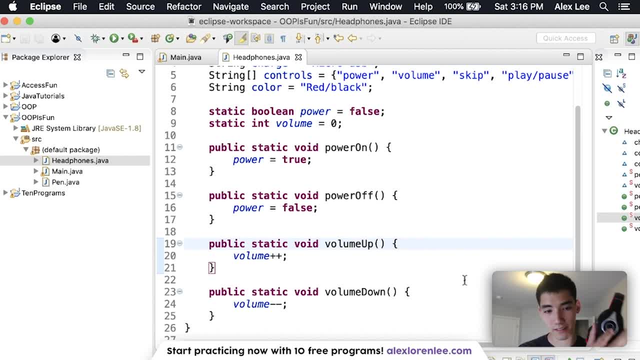 like a state. is a button push the on state or the off state. We know that if it's off then we can't like. the buttons don't work except for the power button. So representing physical objects makes it super awesome to program. 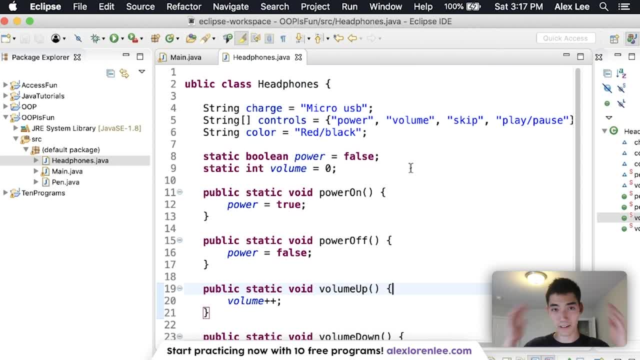 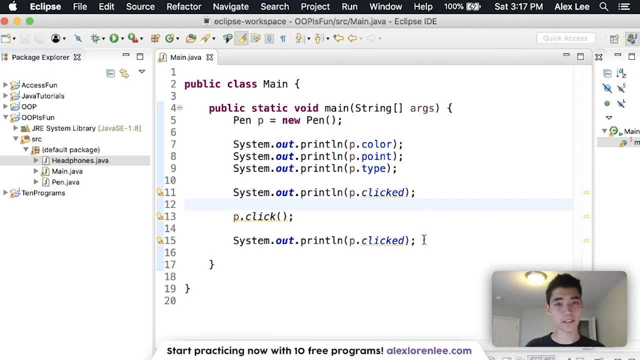 and very easy to keep track of, because you know what it is, you can create a mental image of it and it's got attributes and functions associated with it. So that's really the basis. You can use the headphone class actually for extra credit.